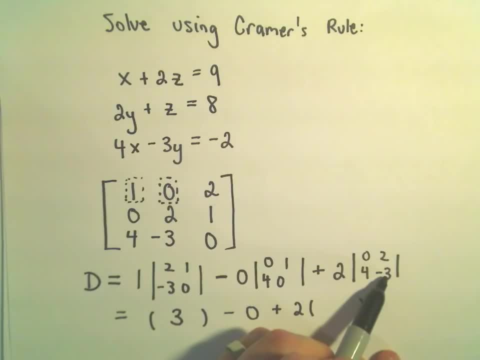 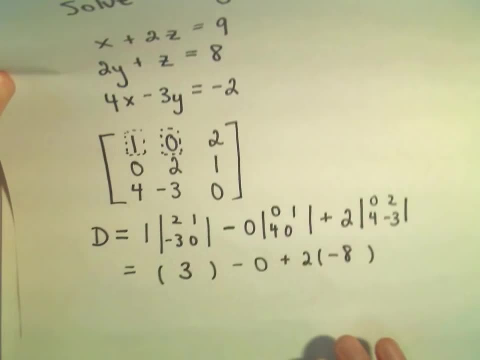 Then we'll have 2 times. Again. it looks like 0 times negative, 3, which is 0.. Minus 4 times 2,, which would be 8.. Alright, so it looks like in this case we're going to get 3.. 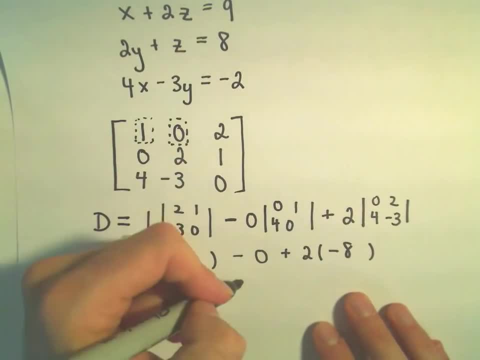 It looks like minus 16.. So if we do 3 minus 16, I'm getting negative 13 for our value for d. Okay, and now this is where we have to go back and compute our other determinants as well. 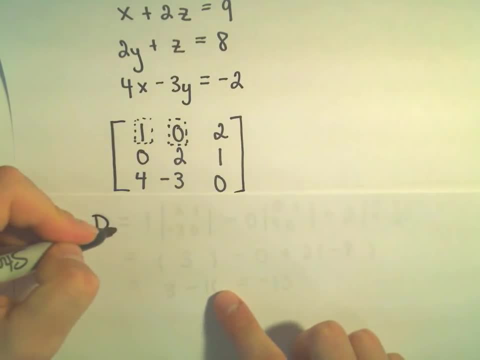 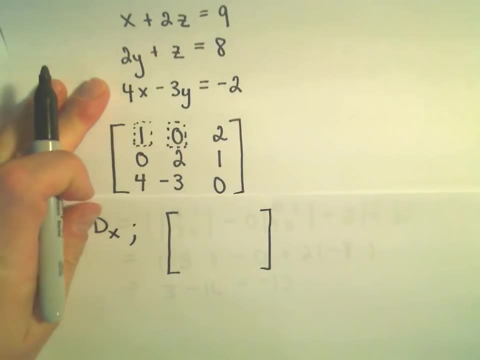 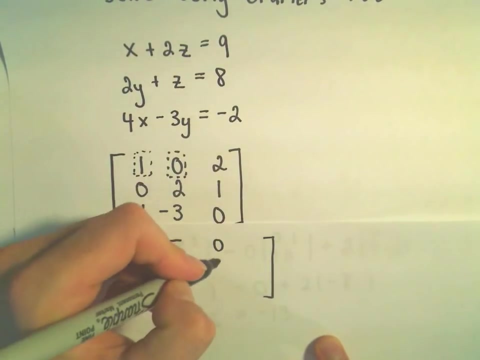 So, to figure out our d sub x, we're going to look at the matrix. So remember, when we do our d sub x, we leave the x column. well, the x column is the one that will change. We leave the other columns alone. 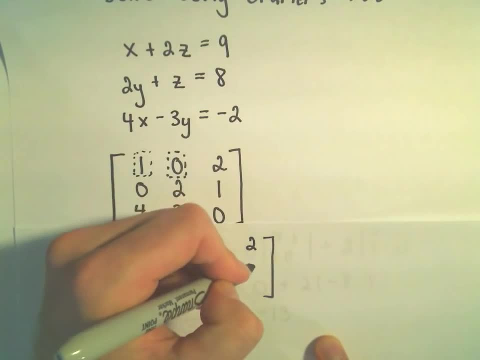 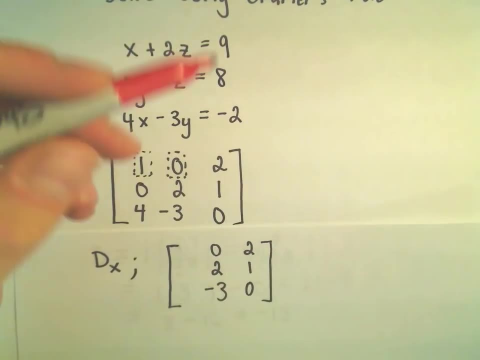 So I'm going to leave the y column alone and I'm going to leave the z column alone And recall: we just take our values that were on the other side of the equal sign, so 9,, 8, and negative 2.. 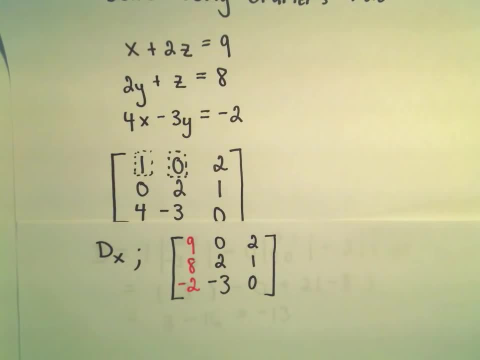 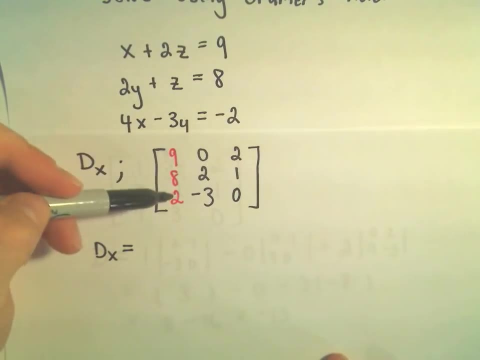 And those are the values that I fill into the matrix. So let's see the same thing. I'm going to do my little determinant, or my, to calculate the determinant, I'm going to expand along the row. So I'm just going to expand along the first row. same thing as before. 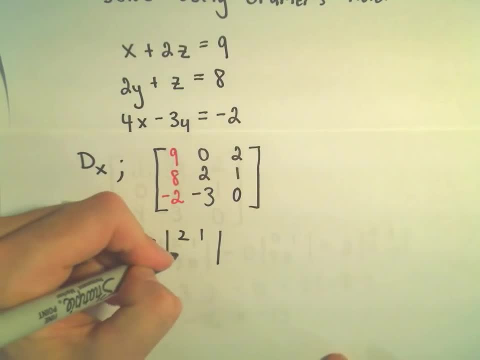 So we'll get 9 times. it looks like 2 and 1 and negative 3 and 0. Then we'll get minus 0 times. well, who cares again, we're just going to get 0 out at the end of it anyway. 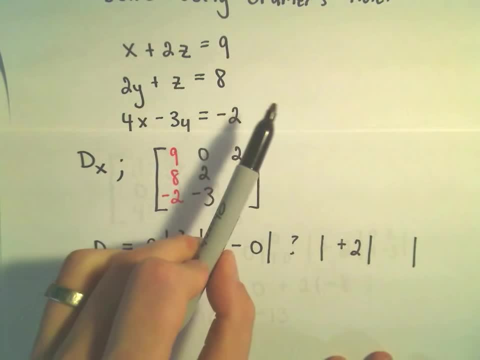 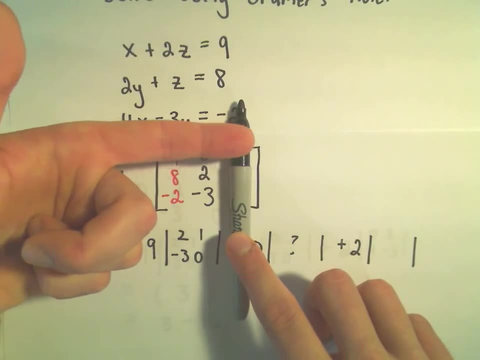 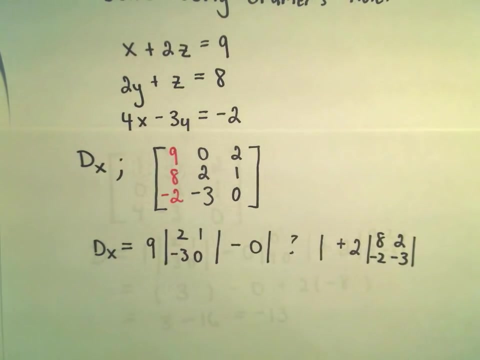 And then we'll get plus 2 times. Let's see, so if I cover up the last column and the first row, it looks like we'll have 8, 2, negative 2, and negative 3 left over. So 8 and 2 and negative 2 and negative 3.. 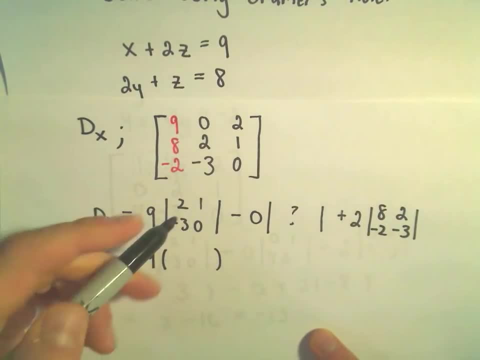 So let's see if we can't do the arithmetic here. So we'll have 2 times 0, which is 0,, minus negative, 3 times 1,, which will give us a positive 3. Our middle term is going to be 0.. 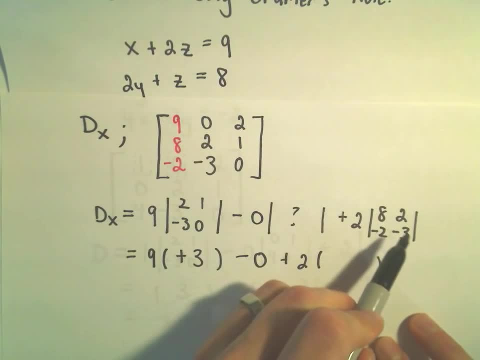 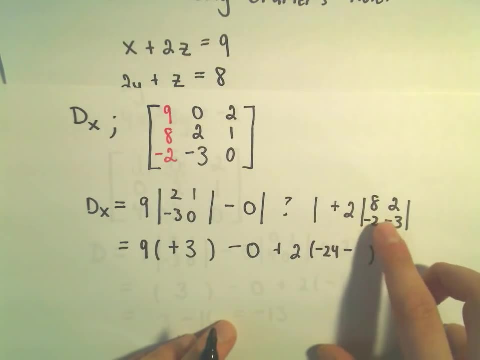 And then we'll have plus 2 times. Let's see It looks like 8 times negative 3,, which is going to be negative 24, minus, let's see, negative 2 times 2 would be negative 4.. 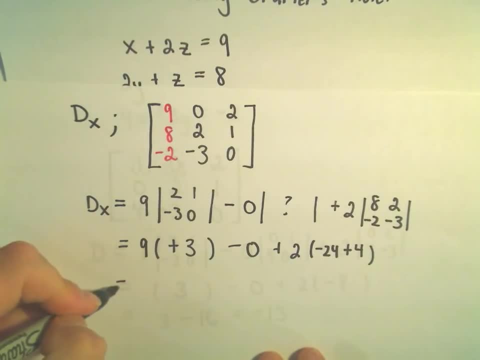 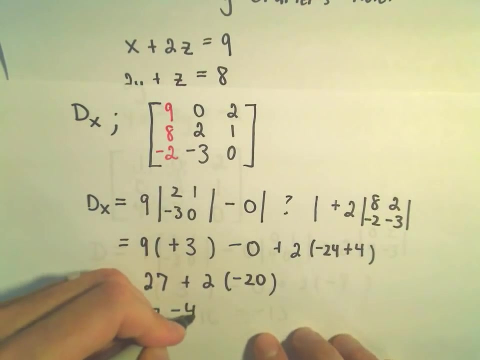 So we'll actually get plus 4.. Well, let's see: 9 times 3 is 27.. Negative 24 plus 4 would be negative 20.. So it looks like we have 27 minus 40. And 27 minus 40 is going to give us a value of negative 13.. 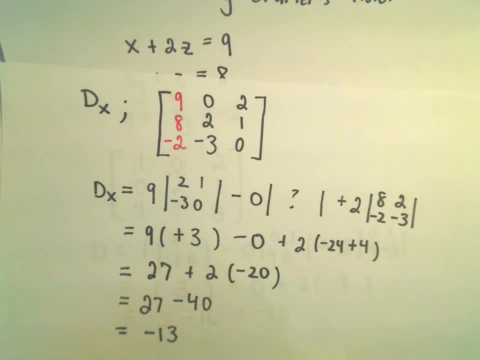 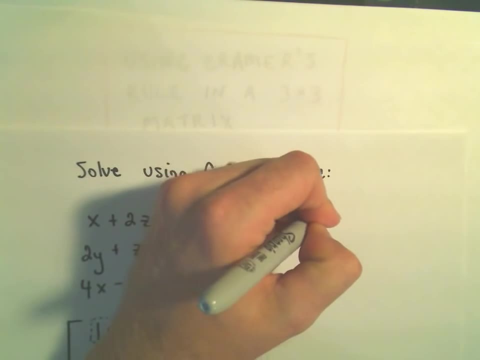 Okay, so there's our d sub x value. So let's see. So we figured out d back here was negative 13.. I'm going to keep them all over here to keep it organized. We now figured out our d sub x value was also negative 13.. 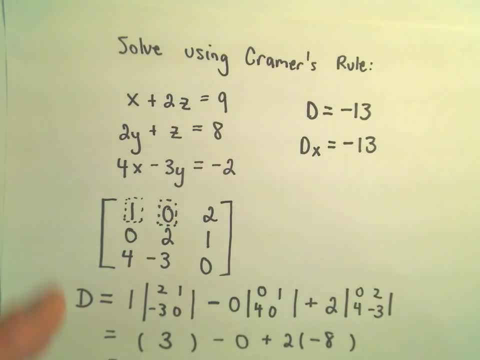 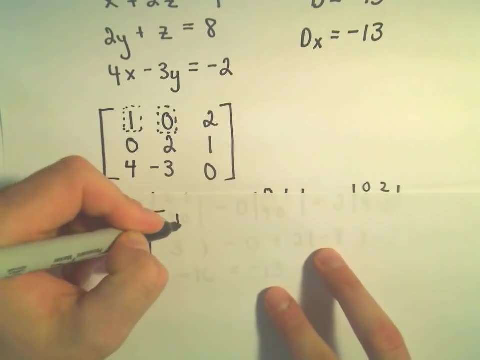 All right, so next we have to compute our little d sub y value. Okay, So to do our d sub y okay again. now I'm going to leave the x column, the original x column alone, so 104.. 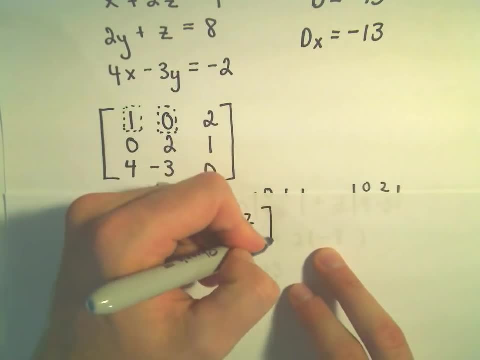 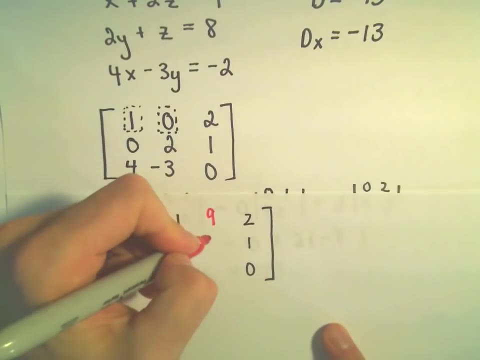 I'm going to leave the z column alone as well, And then again, just like before now, I replace the y column with these values: 9,, 8, and negative 2.. So I'm going to compute my determinant. You could expand along a different row because there's some 0s, but I don't know. 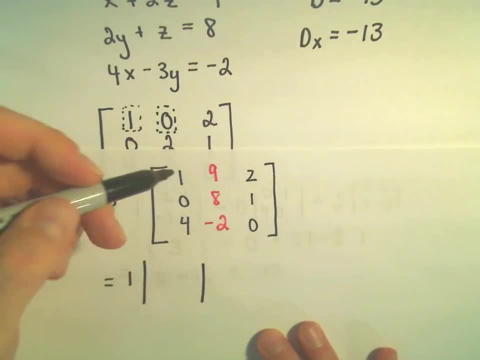 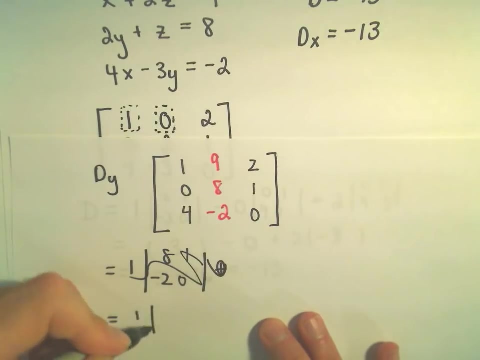 I'm just going to still expand along the first row, So we'll get 1 times. let's see we would get this: 8,, 1, negative, 2, and 0.. Plus, oops, so the middle sign. so we start off with a positive. 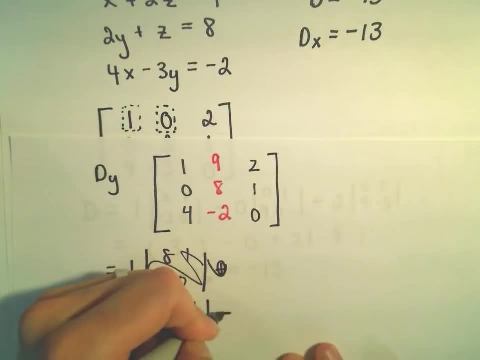 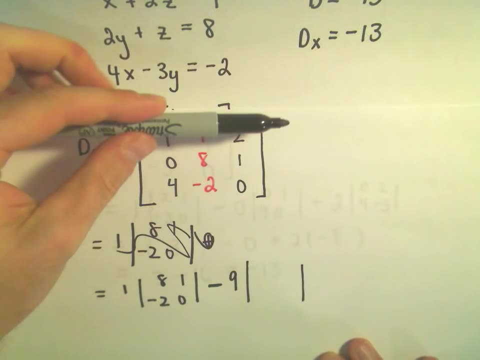 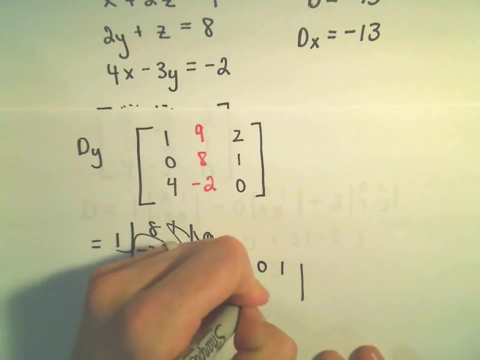 So we have 8,, 1, negative 2, and 0.. The middle sign needs to turn into a negative. We flip the sign So we'll have negative 9. And if we cover up that row and that column, it looks like we have 0,, 1,, 4, and 0 left. 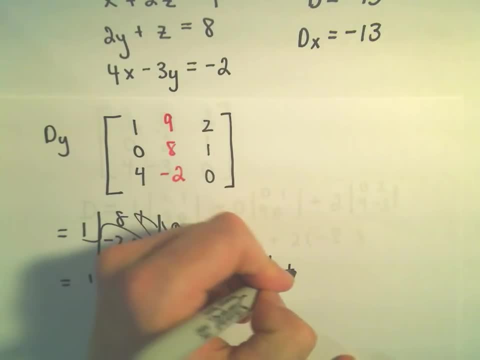 So you can see there's just tons of arithmetic in these. It's certainly easy to make a mistake. Our last entry: we have a positive 2.. We leave that sign positive, It looks like we would get 0 and 8, and then 4 and negative 2.. 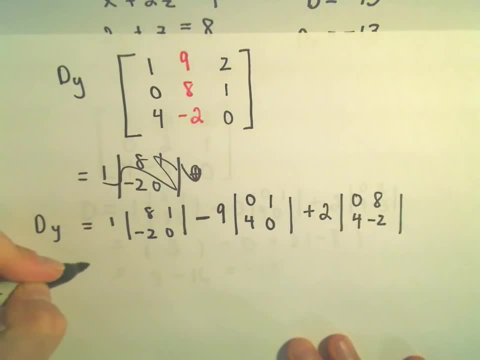 So now, if we compute this, this will be our d sub y. It looks like we'll get 8 times 0, which is 0, minus negative 2, or we'll get a positive 2.. Minus 9 times well, 0 times 0 is 0.. 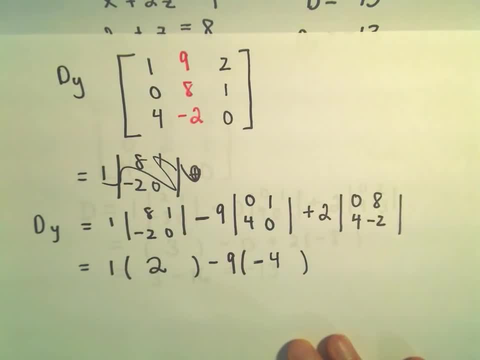 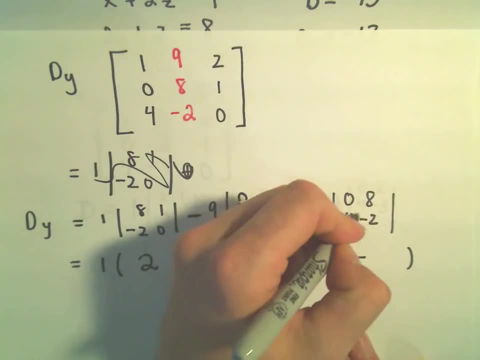 We'll get minus 4 times 1, or negative 4.. And then it looks like we have 2 times well, 0 times negative. 2 is 0, minus 4 times 8,, which would be 32.. 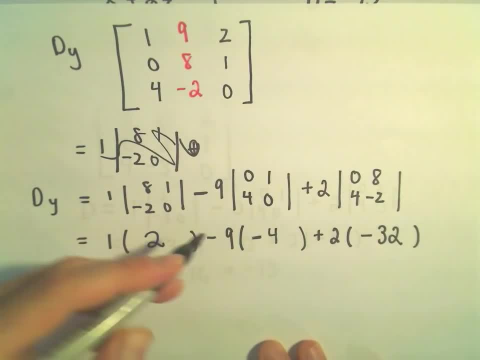 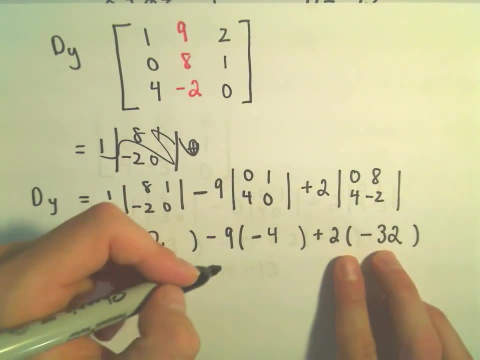 Okay, so if we do the arithmetic here, 1 times 2 is 2.. Negative 9 and negative 4 is positive 36.. It looks like we have positive 2 and negative 32,, which would be negative 64.. 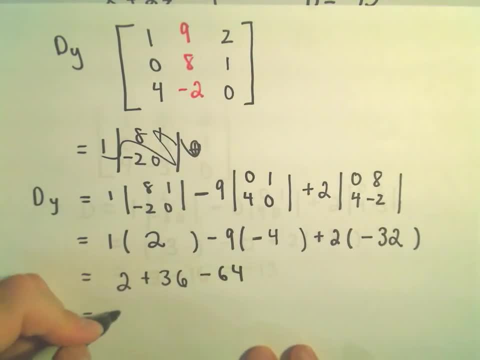 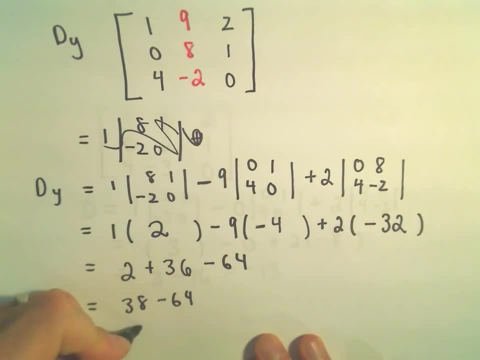 Okay, so let's see what is that. So we've got 38 minus 64.. If we take 38 minus 64, it looks like to me we're going to get negative 26 for our d sub y. So let's see here. 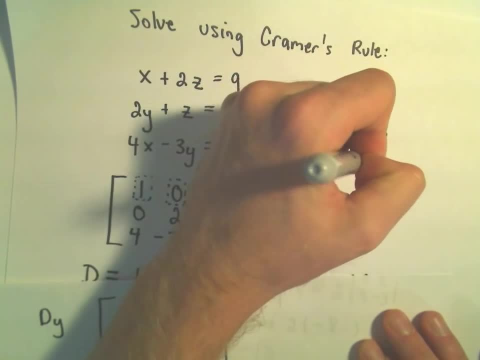 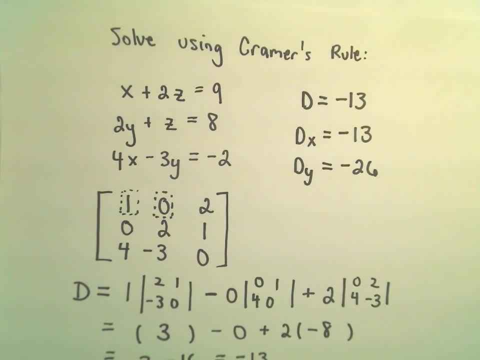 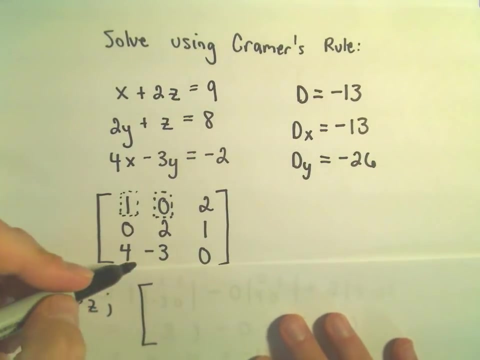 We now have our d sub y to equal negative 26.. So one last one here. We've got to calculate our d sub z value. So to get our d sub z we're going to look at the matrix. So we'll leave the x column alone. 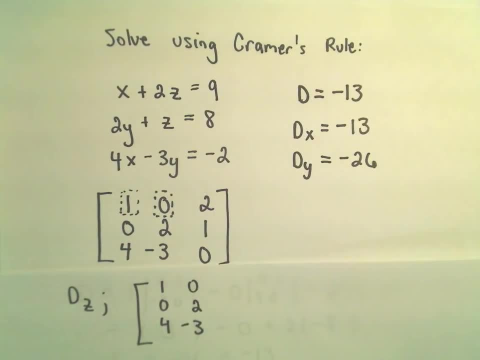 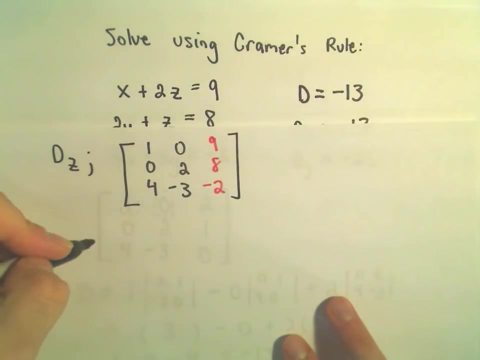 We'll leave the y column alone, And then we're going to in our z column, we'll use these new values of 9,, 8, and negative 26.. Negative 2. And again, we've just got to compute the determinant of this new matrix, coefficient matrix. 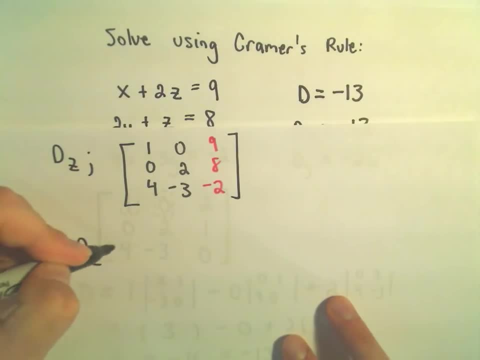 So if we expand along the first row we'll have 1 times. it looks like 2 and 8, negative 3 and negative 2.. We've got to change the sign on the middle, But again we're multiplying by 0.. 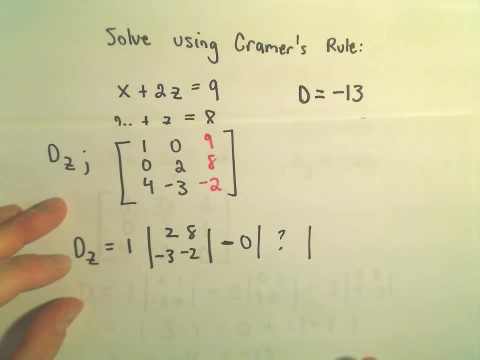 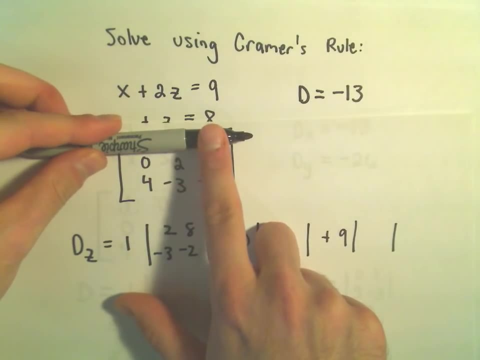 So I don't even bother to figure it out, because I know it's all going to turn into 0 anyway Plus 9.. And then, if we cover up the last row and the last column, it looks like we've got 0,, 2,, 4, and negative 3 left. 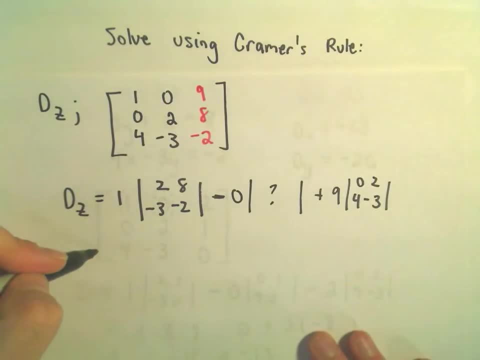 So now we have to compute this last value, So we're having fun here. So 2 times negative 2 is negative 4.. Minus, let's see negative. 3 times 8 would be negative 24.. 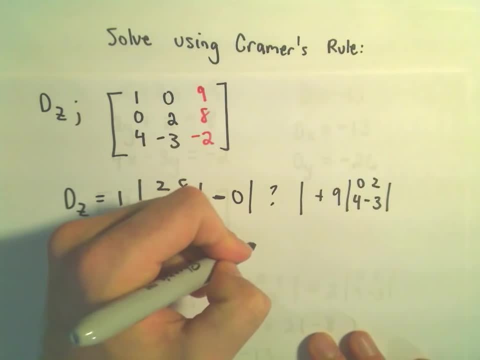 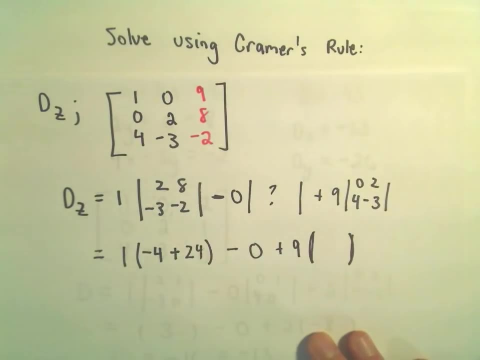 So we'll get a plus 24.. Our middle term is going to be 0. And then we'll have 9 times. okay, whoops. So 0 times 3 would be 0. Minus 4 times 2, which would be 8.. 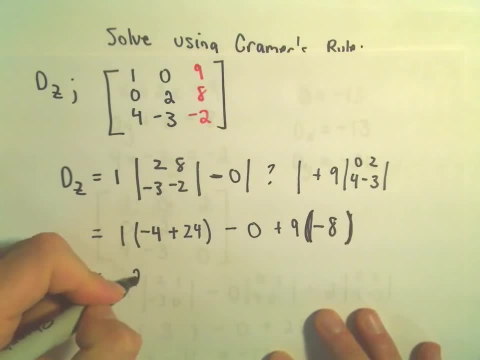 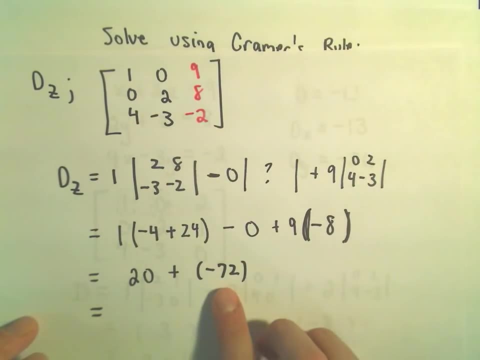 So let's see here It looks like we have negative 4 plus 24,, which would be 20.. Plus, let's see, 9 times negative 8 would be negative 72.. Negative 72 plus 20 is going to be negative 40.. 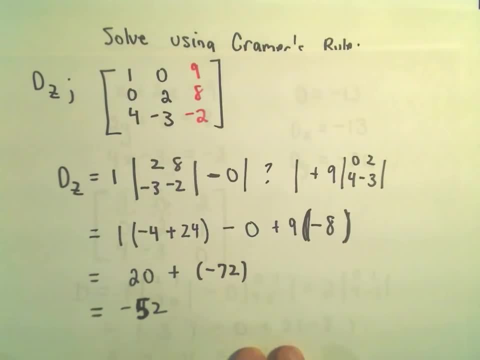 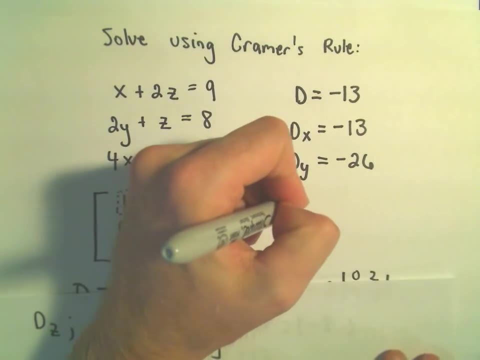 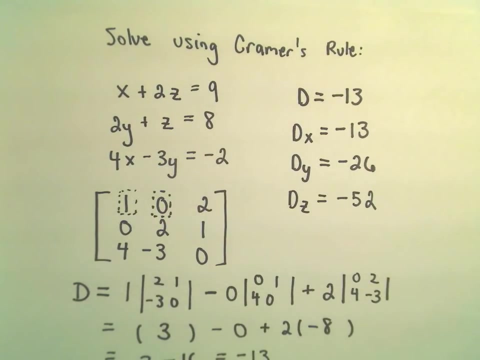 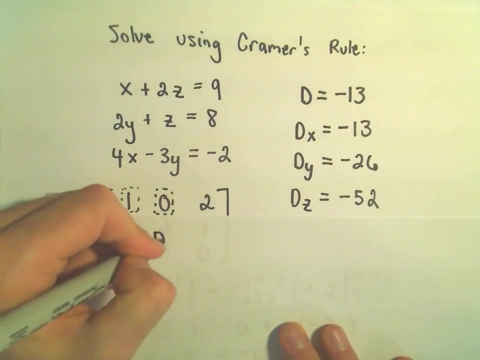 Oh man, How about negative 52?? So now we've got our D sub Z value. So it says D sub Z is going to have the value negative 52. And now all we have to do to actually calculate our solutions again is, it says, to get our final solutions, we take our D sub X over D. 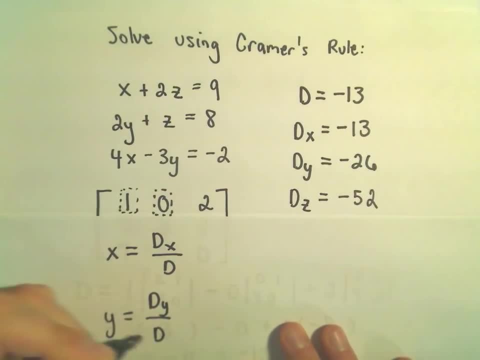 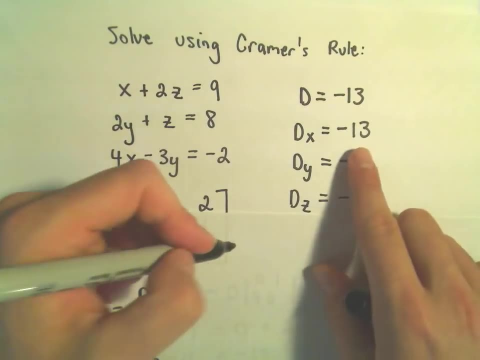 Y is going to be the D sub Y over D, And then our Z is going to be our D sub Z. Well, our D sub X. we got negative 13 over negative 13.. That's going to give me an X value of positive 1.. 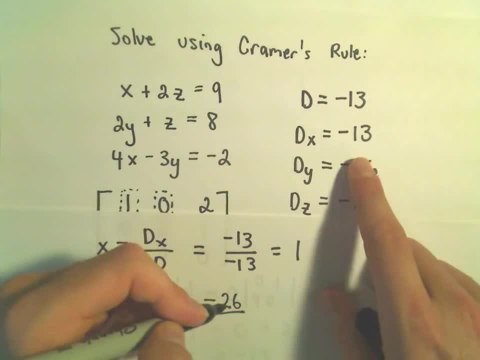 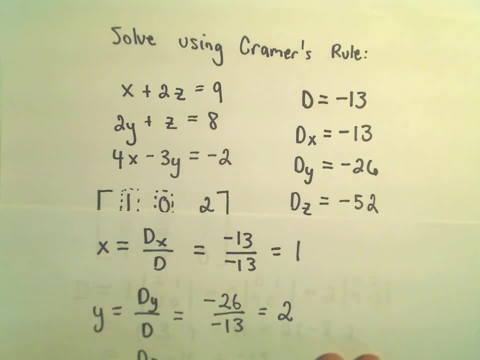 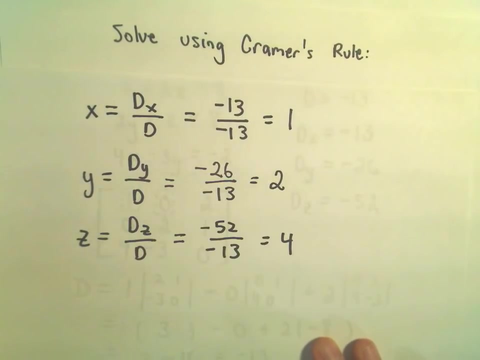 D sub Y is negative 26,, again over negative 13. So negative 26 over negative 13 is positive 2.. Our D sub Z value was negative 52. So negative 52 over negative 13 is positive 4.. 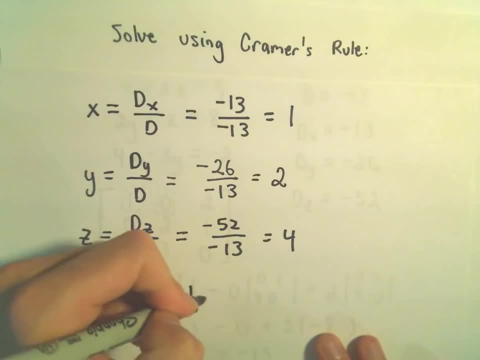 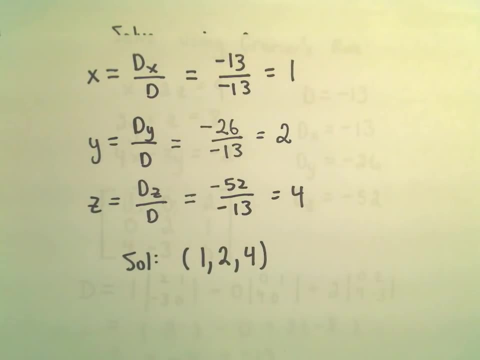 So it says our solution to our original system of equations is 1,, 2, and 4.. So, as you can see, again, pretty long problems. You saw me almost make a couple little mistakes there, So you really have to be a good bookkeeper on these problems. 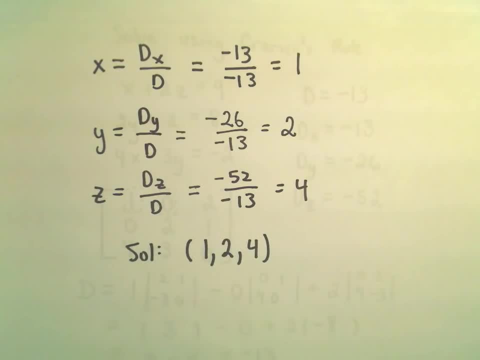 You know, if you miss one little computation, one little sign, one little, any one little arithmetical mistake by the time you get to the end of it, obviously you know you're going to be off by a good bit.